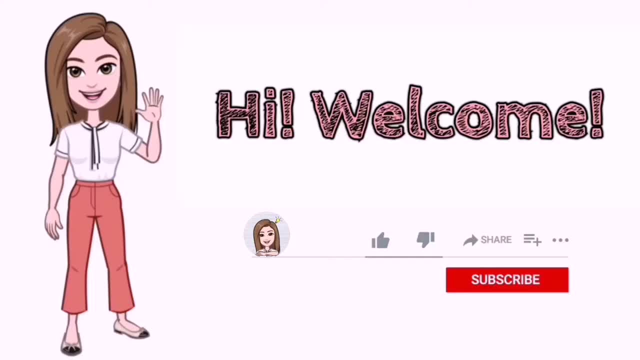 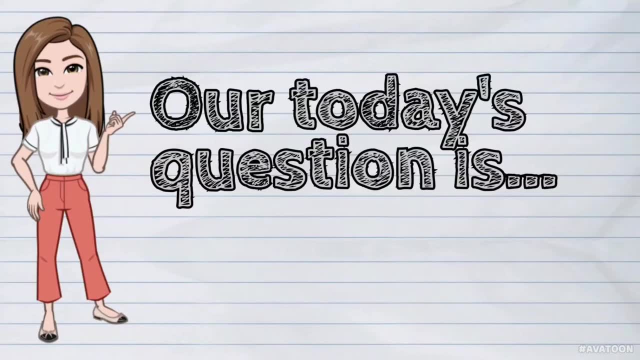 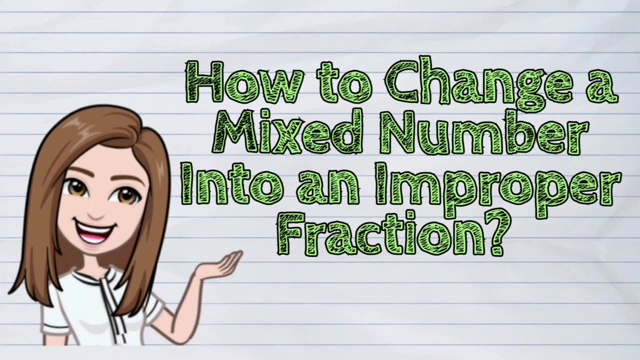 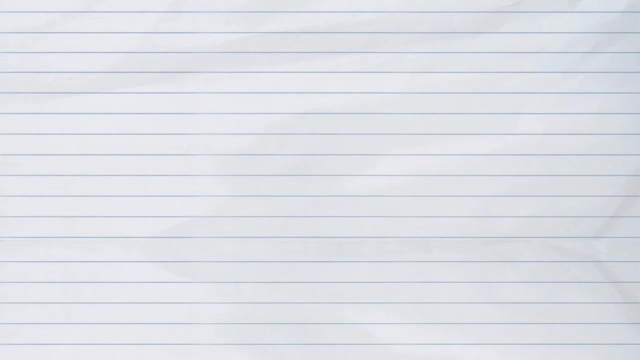 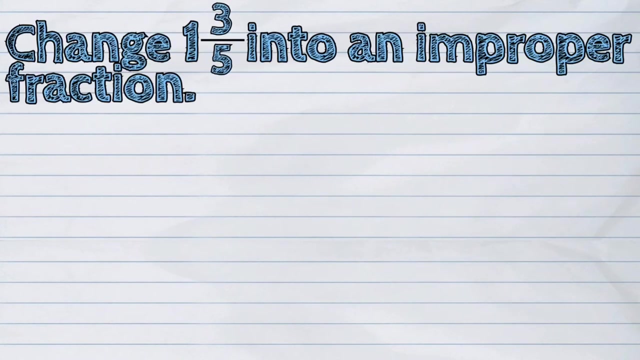 Hi, Welcome to iQuestion PH. Our today's question is How to change a mixed number into an improper fraction. To learn how to change a mixed number into an improper fraction, let us study this example: Change 1 and 3 fifths into an improper fraction. 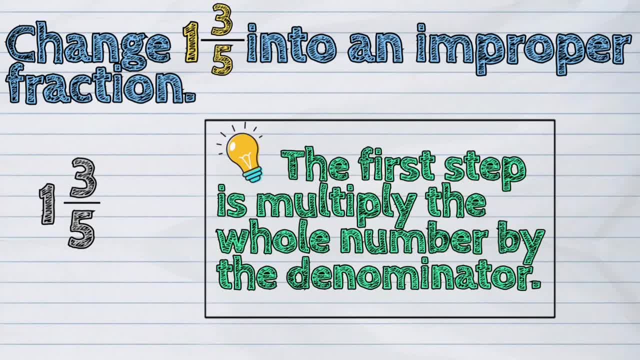 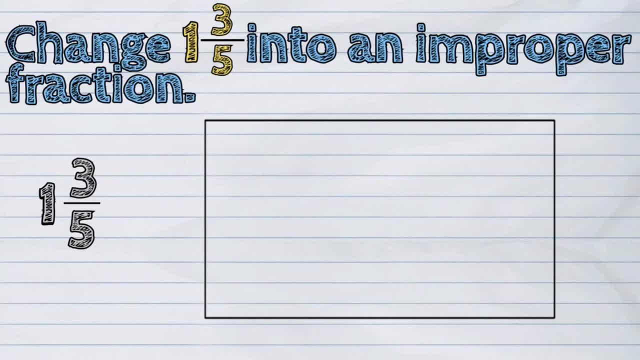 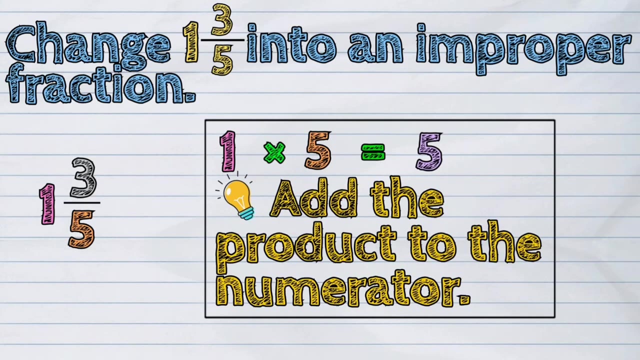 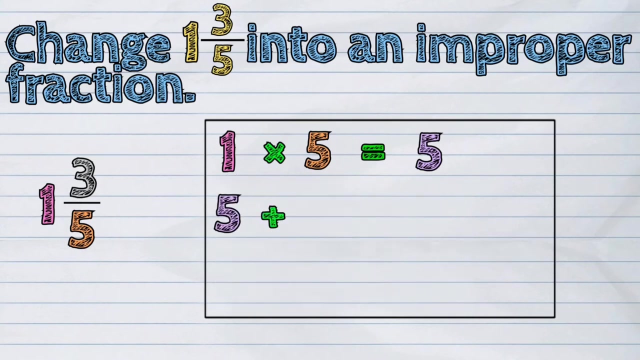 The first step is multiply the whole number by the denominator. In this case it's. The answer here is Then: add the product to the numerator: Our product, which is 5, plus the numerator, which is 3.. This gives the answer of: 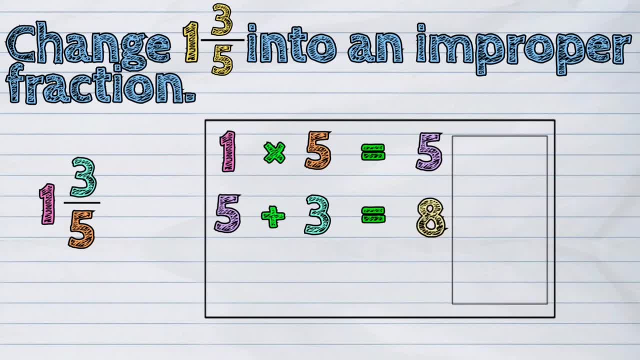 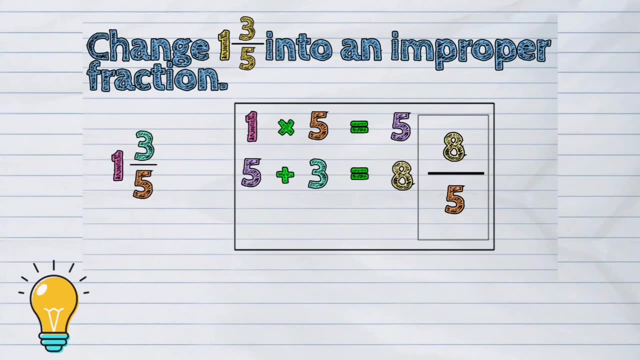 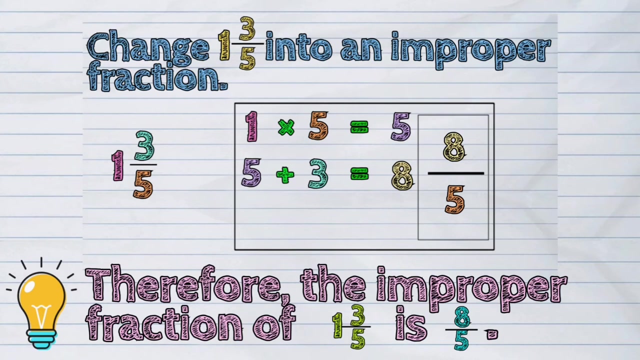 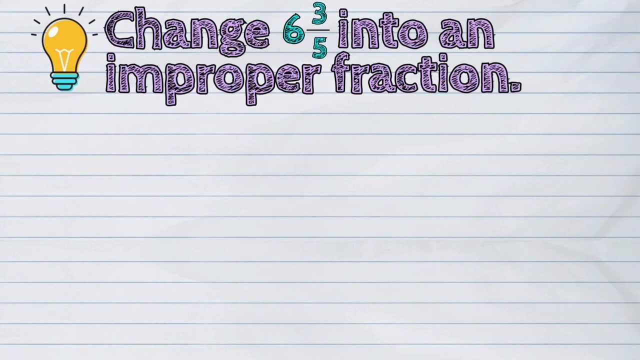 The 8 here. Here will be our numerator And we are just going to copy the denominator in our mixed number, which is 5.. Therefore, the improper fraction of 1 and 3 fifths is 8 fifths. Let's have another example. 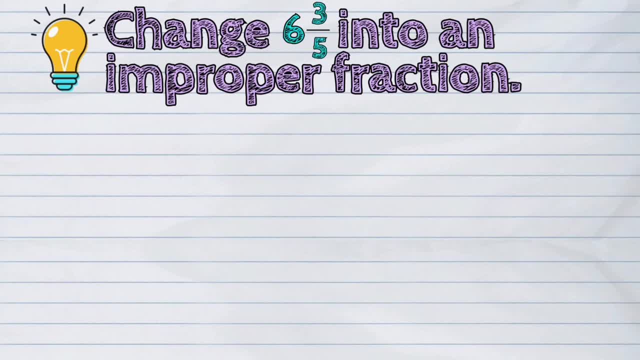 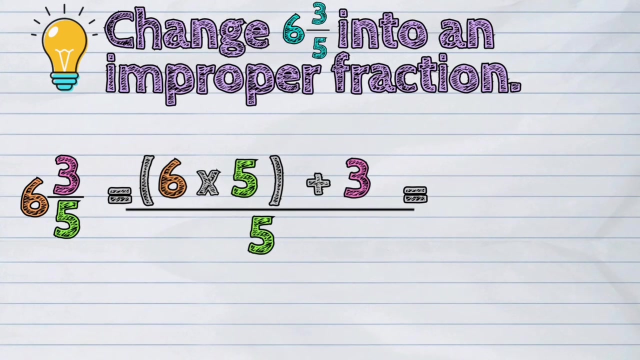 Change 6 and 3 fifths into an improper fraction. Again, the first step is to multiply the whole number by the denominator. Next add the product to the numerator, Then write the answer on top of the denominator. So 6 times 5 is